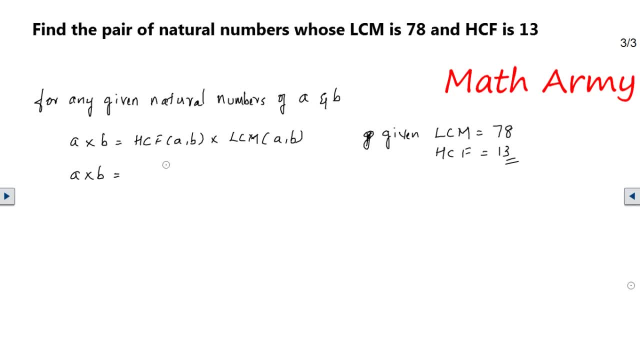 So one and the same. And now, so what is the product of 13 and 78? It is 1014.. Now, so do a prime factorization of 1014 and you will be getting 2,, 3,, 13 and 13 as your factors. 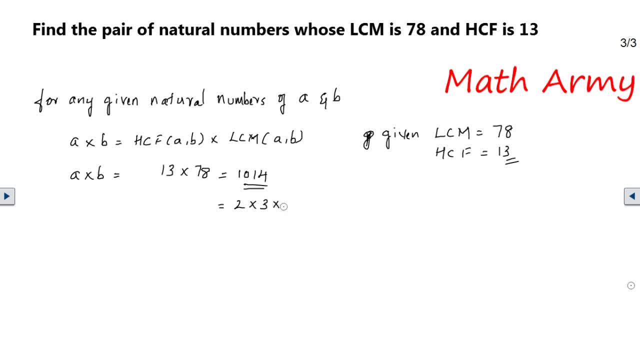 So, therefore, 2 multiplied with 3, multiplied with 13 and multiplied with again 13.. You'll be getting a product of 1014.. So let us cross check once. Okay, With 2.. 2,, 5,, 0,, 7 times. 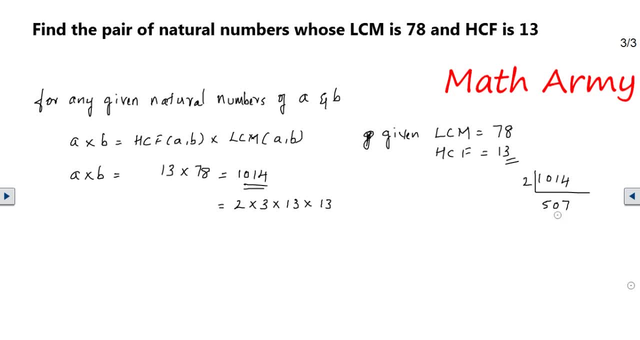 Right, Yes, And he divides 3, 1 times 6 times and 9 times 3 divides 507 in 169.. And what is the Next prime number? 13.. 13 divides 169, 13 times. 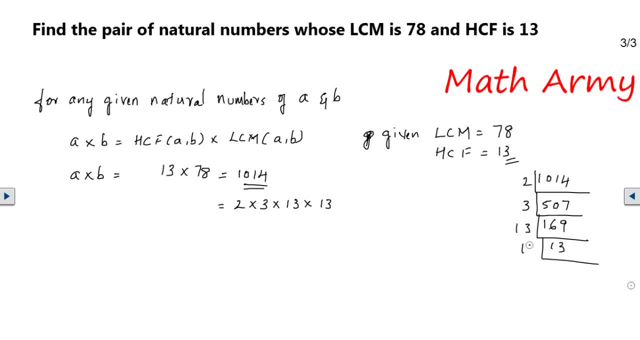 And 13 divides 13, 1 time. So therefore, 2 multiplied with 3, multiplied with 13 and 13 gives you 1014.. Just, I cross checked on the right hand side, So we are good with that. 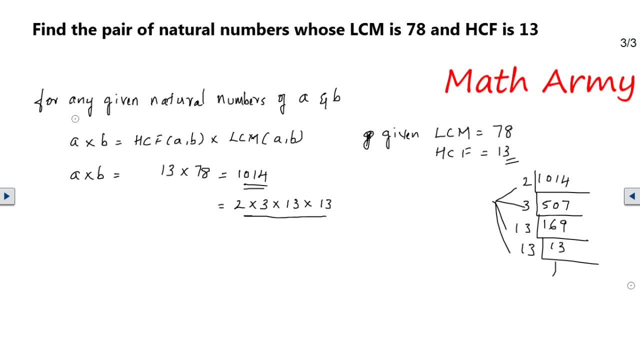 And now what these people are saying, Guys, and what is the highest factor among 2,, 3,, 13 and 13?? It is 13,, right, And what actually given in the question, HCF as 13.. 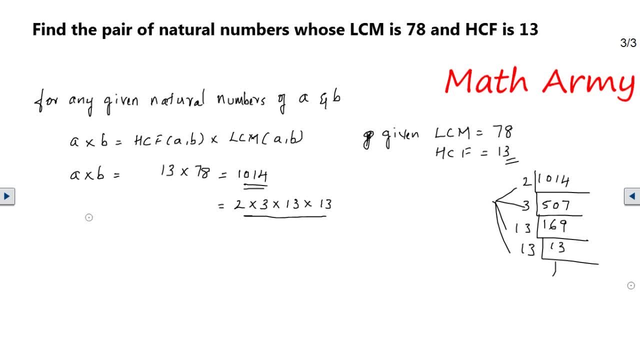 So you can safely say that 13 is our HCF And that is what understood. Since 13 is HCF, 13 should be the multiple of the numbers. Yes, So 13 should be the multiple of the given numbers. 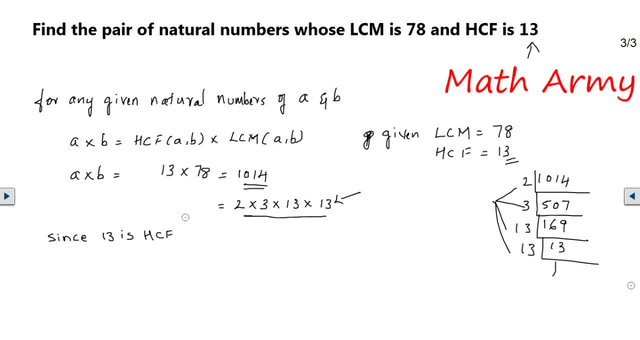 What are the given numbers? We don't know. So one number would be A and second number would be B. So what we are supposed to do? The same A multiplied with B. It is 2 into 3, into 13, into 13.. 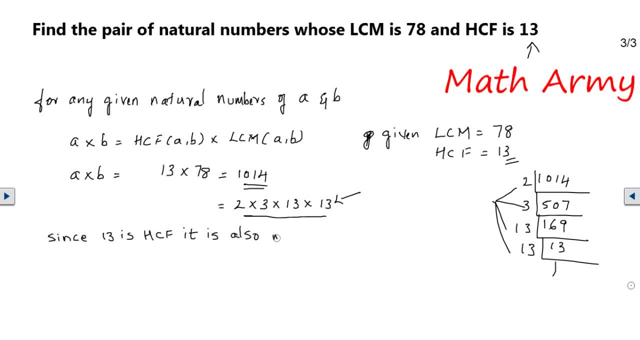 Let us reframe a little bit, Okay, And what happens? So same 2,, 3,, 13,, 13.. I am going to rearrange them. See how I am going to: A into B is equal to 2 multiplied with 13 is going to be one pair.